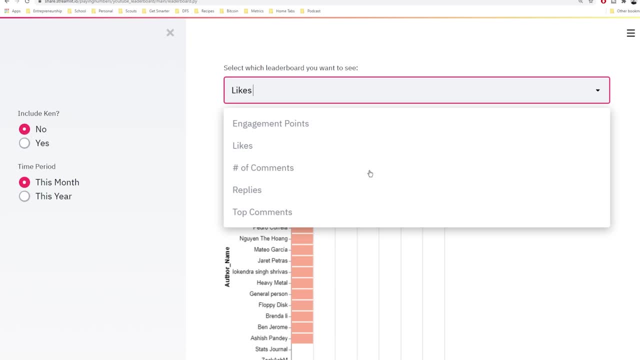 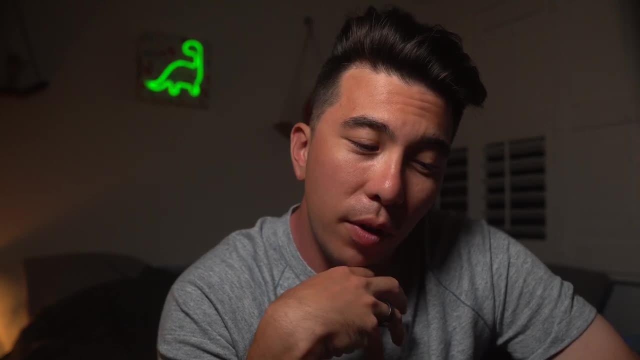 A great example of this is my leaderboard project for my YouTube channel. I was able to get all the comments on my channel from YouTube's API. I've also linked a few resources below with some public data APIs that might be of interest to you. Most of the data that you're working with in the field. 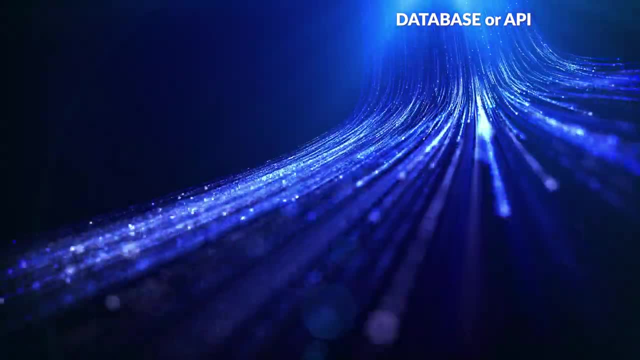 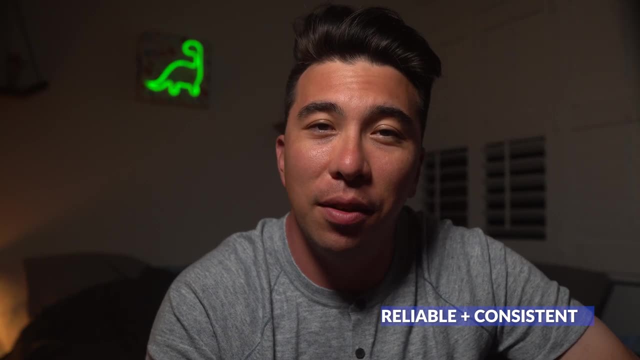 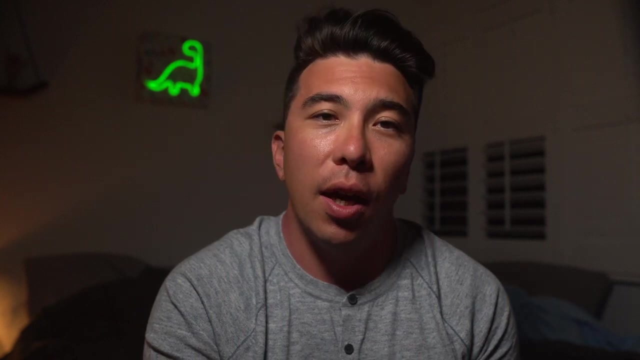 is either coming from a database or from an API. You may even be accessing your databases from an API as well. As we mentioned, APIs are meant to be reliable and consistent, and accessing or creating an API can be part of the data pipeline. Now, data scientists don't just use APIs. we 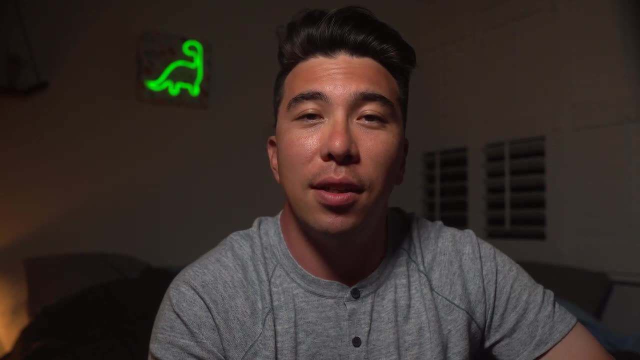 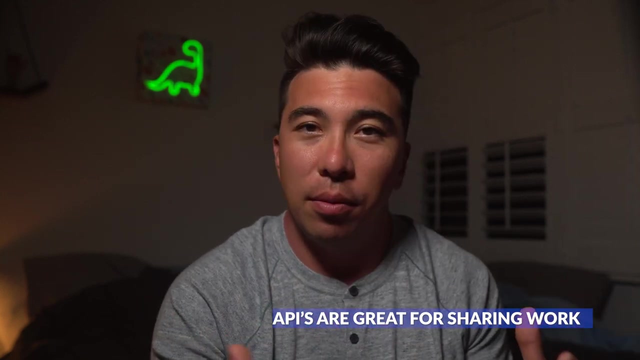 also create them. In many companies, the main products that data scientists produce are, in fact, APIs. You're probably thinking, but I thought data scientists built models and made beautiful visuals. You're definitely right on that front. However, one of the best ways to make your model 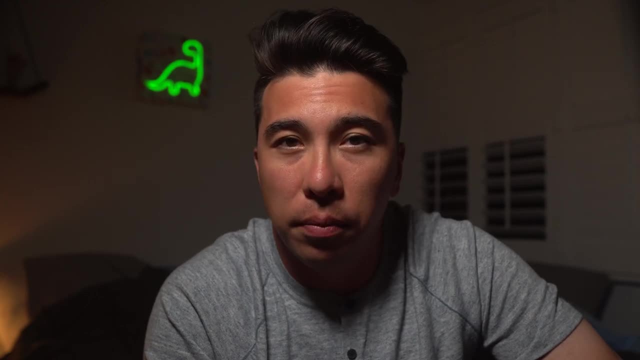 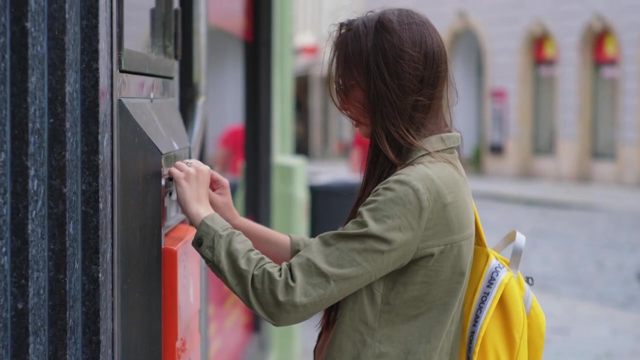 usable to other people is to turn it into an API endpoint. With that, software developers or even other data scientists can send data to your API and they'll in turn receive the results of your machine learning model. I'm sure that the models you're building 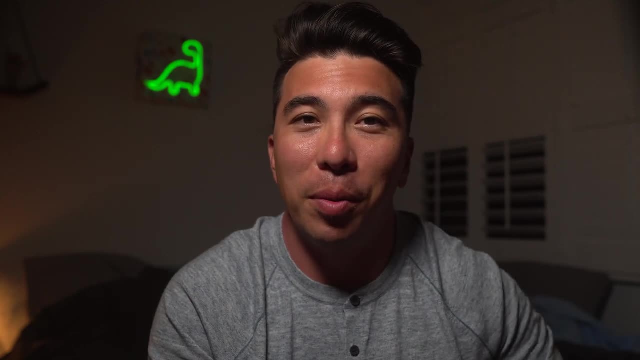 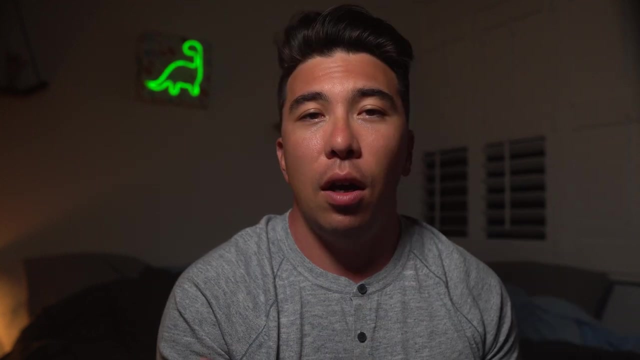 are great, but they're completely useless unless they can be used by other people. The last big way that APIs are useful to data scientists is by leveraging other people's models or services. Often someone else might have a model that we want to use in the pipeline. 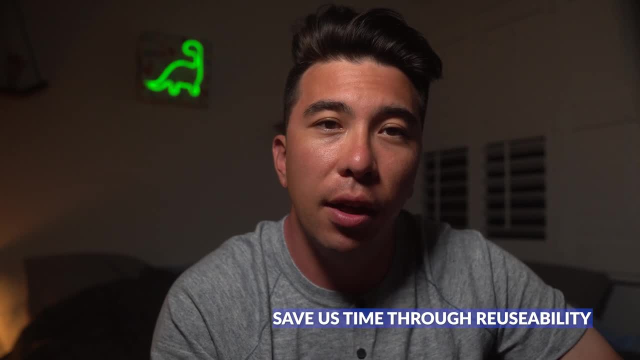 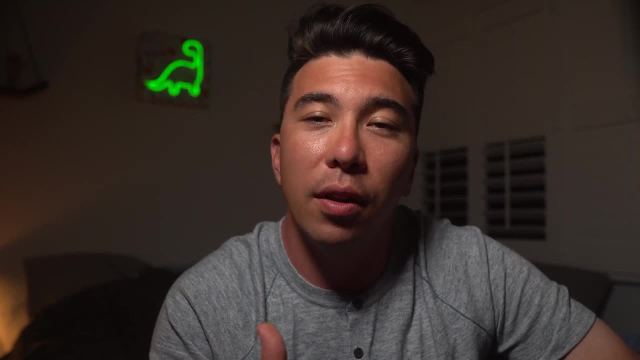 of our work. Instead of downloading their code and recreating it, I can just leverage the API that they've already created. As a data scientist, I can also use APIs to implement the work that I've already done. For example, through the Twitter API, I can post a tweet If I built. 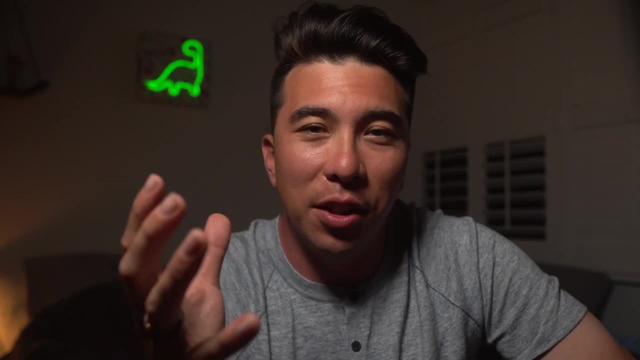 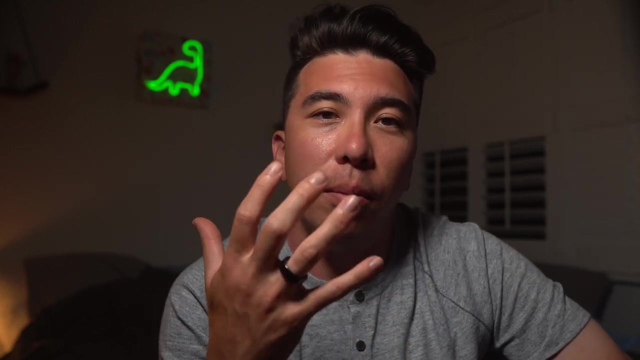 a sick machine learning model that collected all of the data on a specific topic, say the 66 days of data initiative. I could have my pipeline directly post that tweet to my account using the API. There are some other uses for APIs, but I think I hit the big ones. 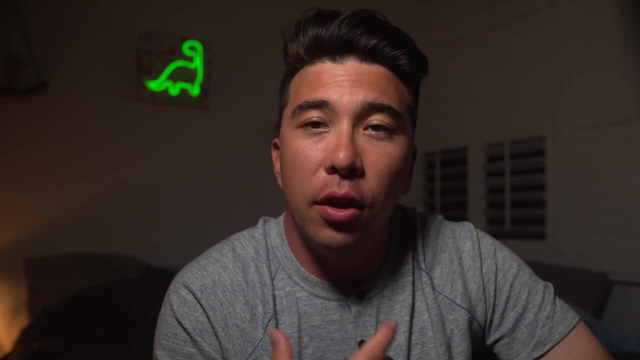 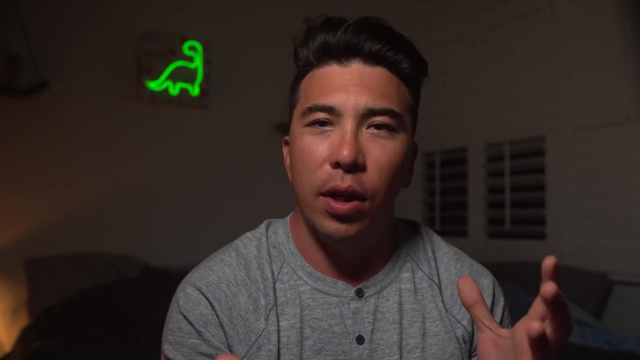 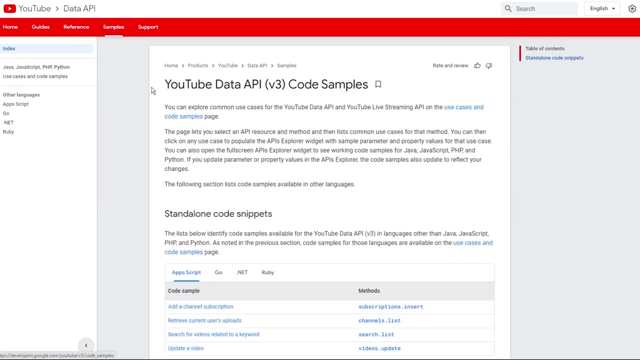 for the data science perspective in this video so far. Your next question is likely: how do I use an API? All APIs follow a fairly similar structure, but they can have their own idiosyncrasies. I recommend finding the documentation for any API you're interested in using and follow the examples that are shown Once you've used a.